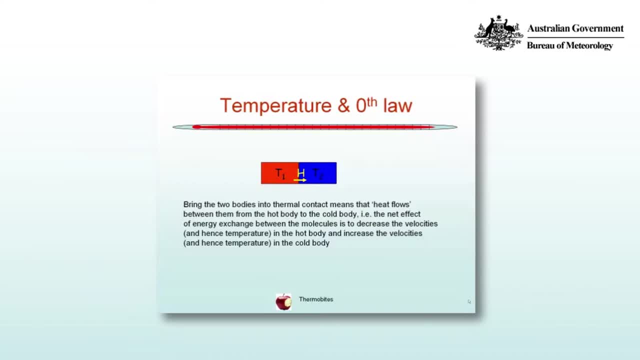 energy exchange in the case of heat flow, and that's a measure of how the molecules interact. So in the hot body with a large temperature there's going to be a greater velocity or the value of the velocity distribution is larger than the cold body. So the net result will be that molecules in the hot body will exchange energy with. 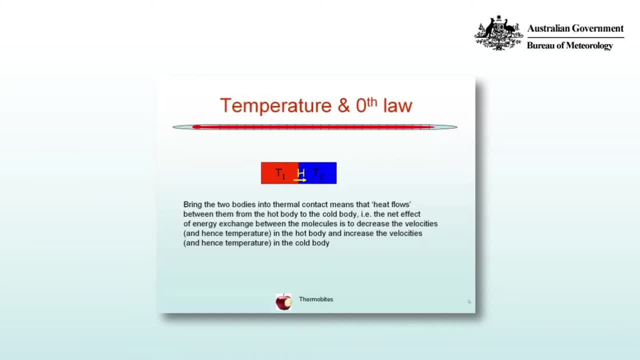 molecules in the cold body such that the energy content of the hot body will go down and the energy content of the cold body will go up, and that will be measured in terms of the temperature. So expect the hot body's temperature to decrease and the cold body's temperature to increase. When we do that, what we can. 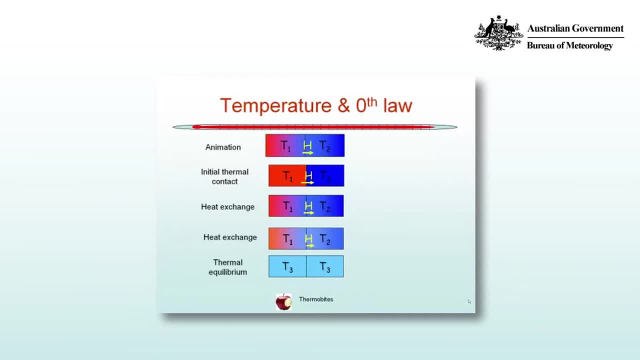 see is eventually that we will get thermal equilibrium, that is, the. the two bodies that are now in thermal contact will have the same distribution of molecular energies and we can measure that in terms of this macro quantity: temperature. so T3 will be less than T1 but greater than T2. And you can see over time the heat exchange. 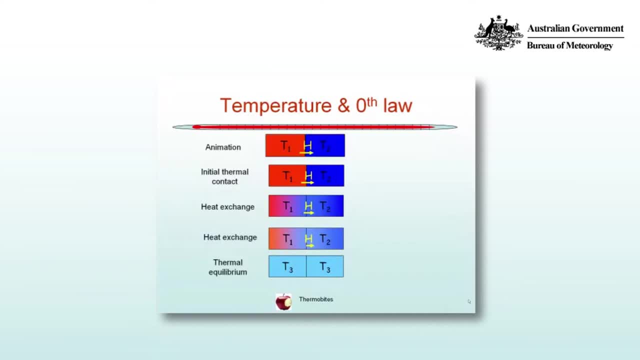 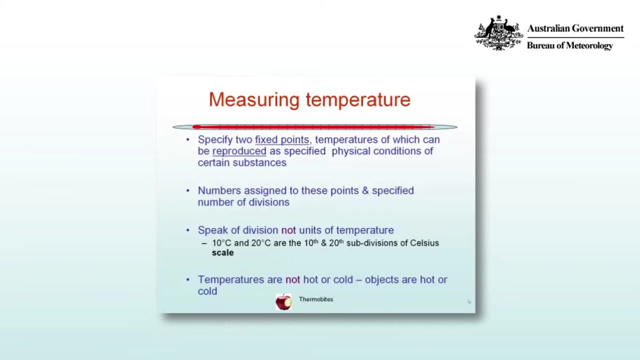 or the energy exchange between the hot body and the cold body decreases until it's essentially a net transfer of zero across the interface between these two bodies. As we discussed before, we measure temperature in terms of a scale, So specify two fixed points. They're temperatures which can be reproduced as specified physical conditions. 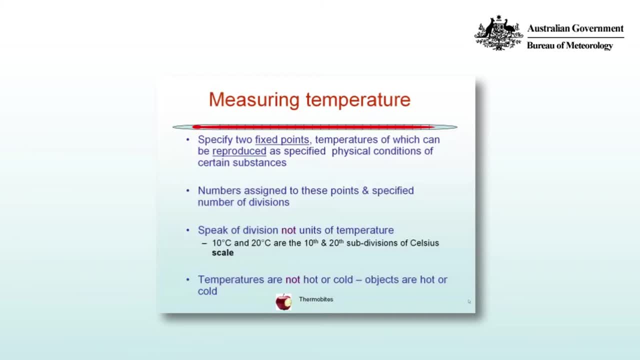 of certain substances And in terms of water, for example, it's boiling and freezing. The numbers are assigned to these two points and then you specify the number of divisions between the two points. So, for example, in Celsius you have zero. is freezing, boiling? 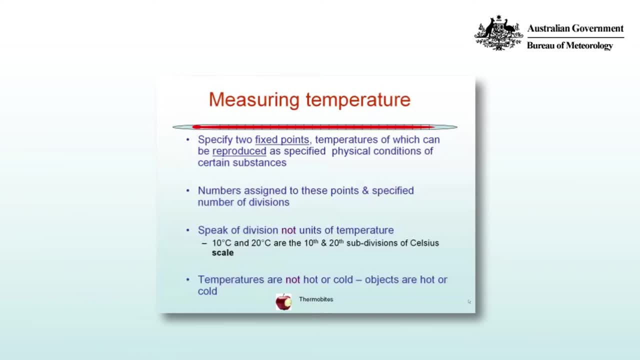 is 100 degrees and then you divide through by 100 to get one degree Celsius increments. So we must speak of divisions and not of units of temperature per se. So, for example, 20 kilograms is twice as heavy as 10 kilograms. 20 meters is twice as long as 10 meters. But